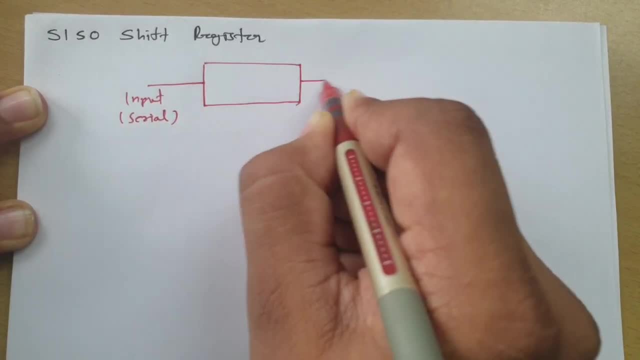 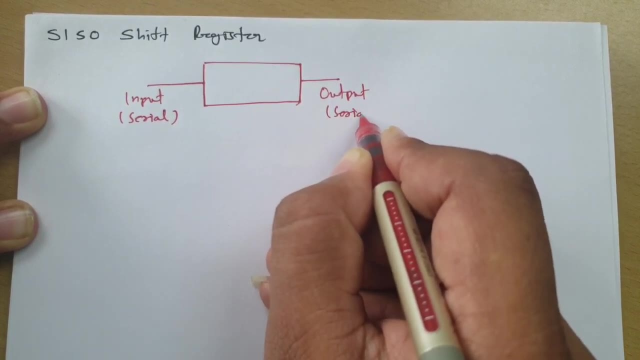 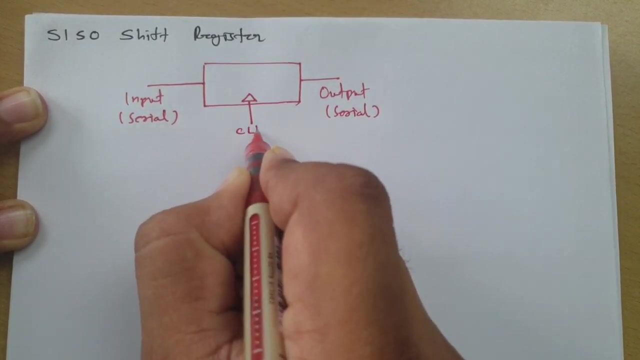 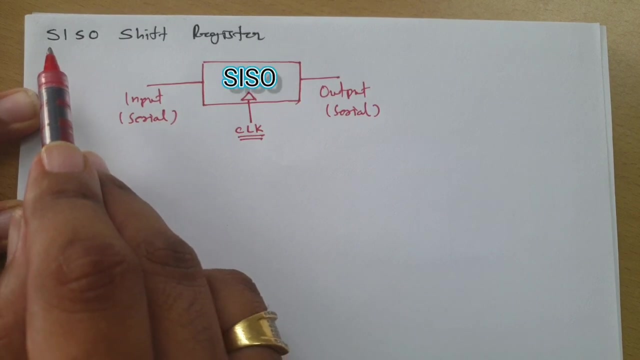 serial input and here there is one terminal which is there at output, and at this terminal we will be taking serial output and this output that will come with respect to clock signal, right. So here, if you see this basic block diagram of serial input, serial output, then there is only one input terminal, there is only one output terminal and 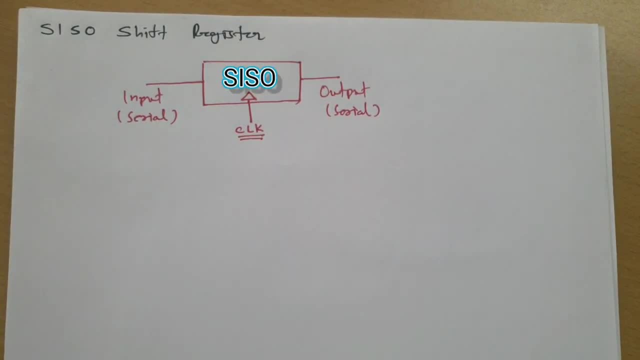 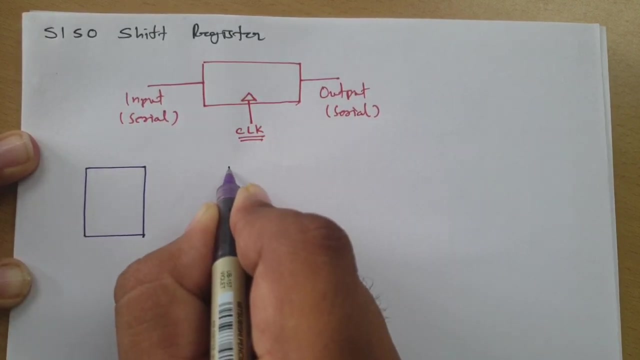 one clock signal. Now here to explain serial input, serial output, shift resistor. here I'll consider 4-bit shift resistor, So shift resistor that we usually made it by having D flip-flop right. So here let me draw D flip-flop here. So for 4-bit shift resistor I'll be using 4D flip-flop. 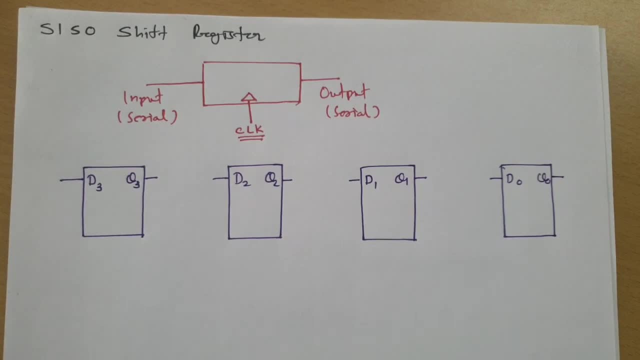 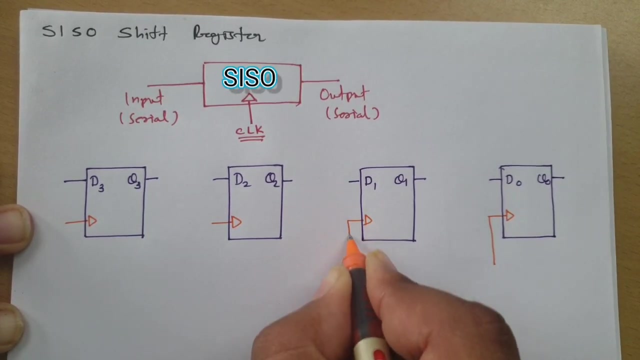 So these are my 4-bit shift resistor D flip-flop right and here I'll be connecting common clock with all 4D flip-flop. So let me connect 4 positive H trigger clock commonly to all 4D flip-flop. 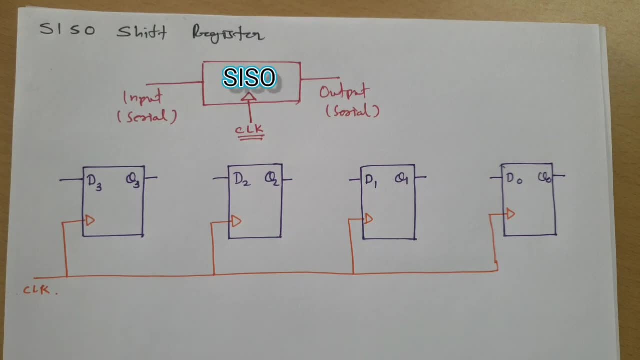 Now here I'll be going to explain you how this serial input, serial output shift resistor is there in its connection. So first I'll explain you how we can have shift right connection. So to have shift right connection we just need to connect Q3 with D2, Q2 with D1 and Q1 with D0.. So in that case 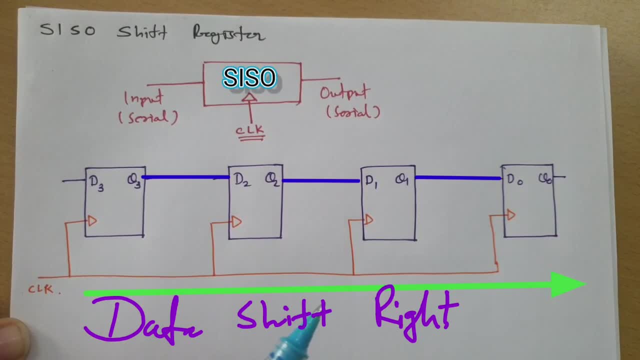 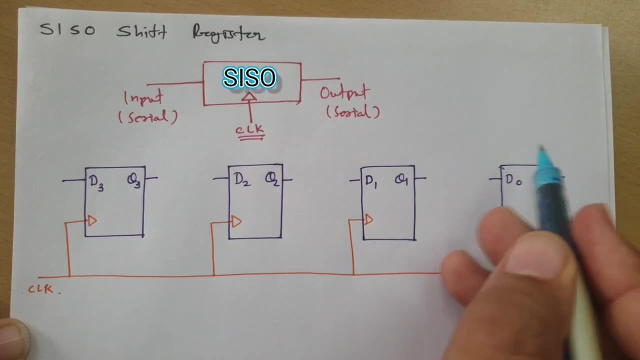 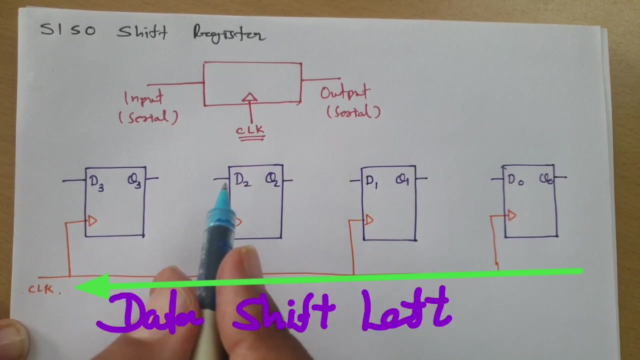 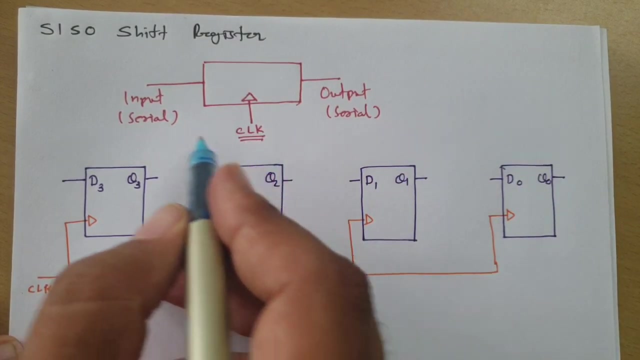 data will get shifted in this direction. that is shift right direction. and we can have even shift left connection In that we need to connect Q0 with D1, Q1 with D2 and Q3 at output side right. So for shift left connection we need to connect Q0 with D1, Q1 with D2 and Q2 with D3. 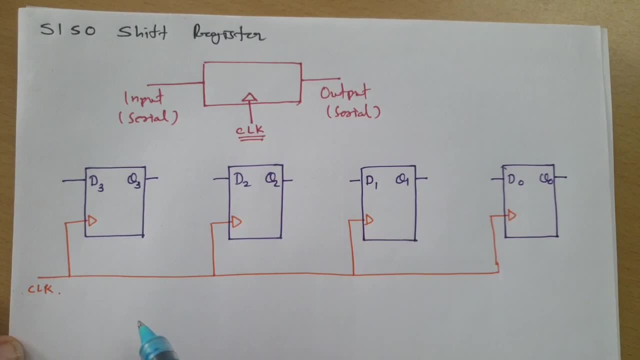 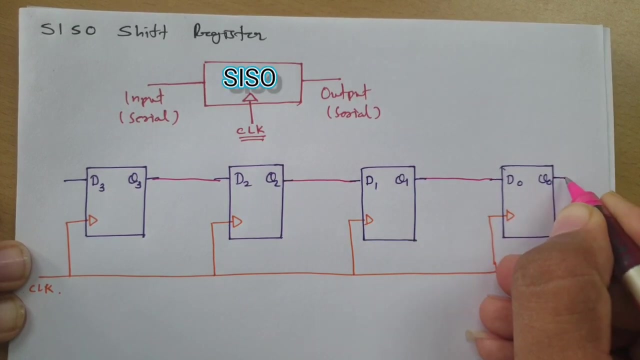 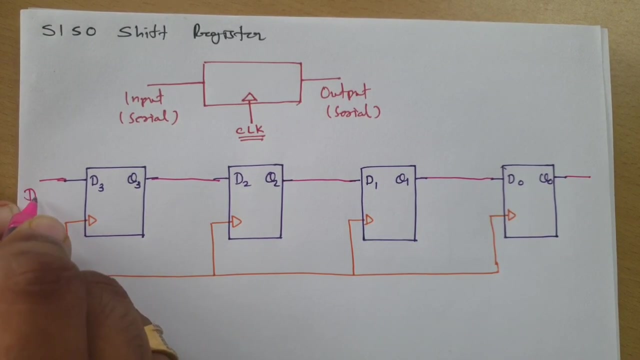 to have shift left operation of shift resistor right. So here I'll explain you shift right connection, and for that I need to have this connection. So this is what the basic circuit which we have, and in this here we have serial input and here we have serial output right. So if you observe this complete circuit package, then that is what this. 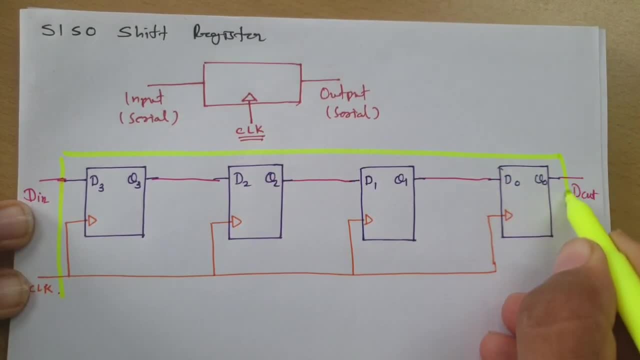 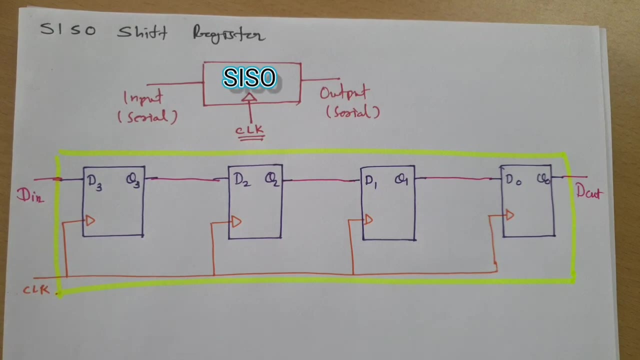 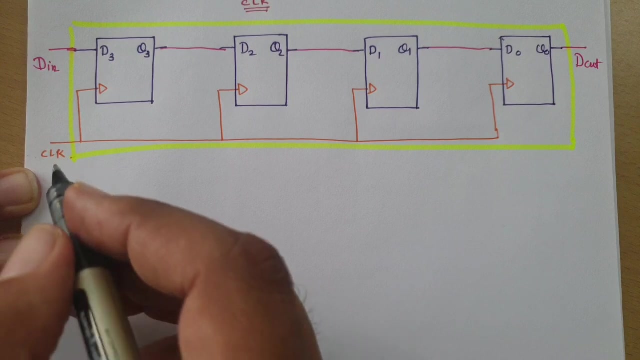 block diagram right, Where only three terminals that we have: input, output and clock D in clock and output, But internally you'll be finding there are four D flip flops. So this is what four bits shift right, register right, And here I'll explain you now how this register functions. So for that here we'll be inserting: 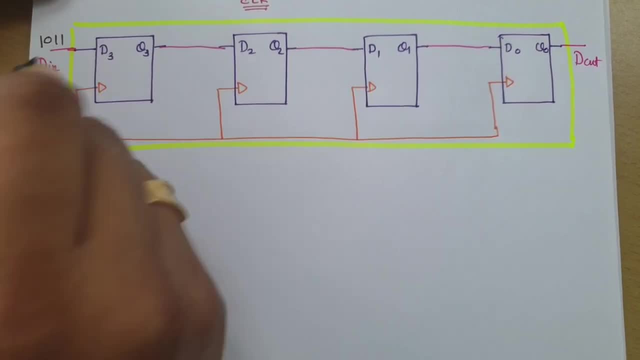 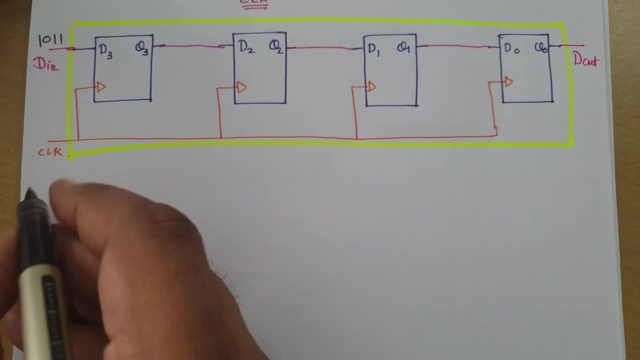 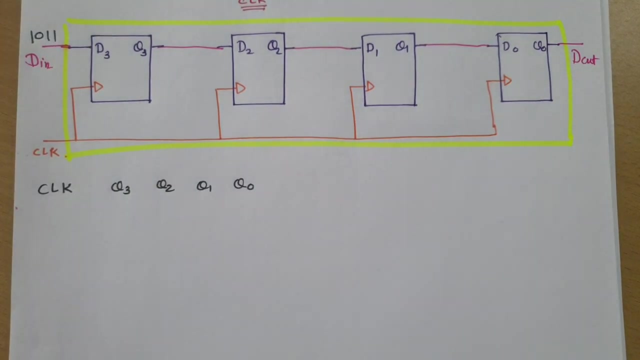 one zero, two, one one data serially and with respect to clock, how that is getting shifted in this direction. That is what we are going to understand. So to understand this data, here I'm writing this is clock signal: Q3, Q2, Q1 and Q0.. That is how output of flip flop is there And initially we are considering all data of output of flip flop. 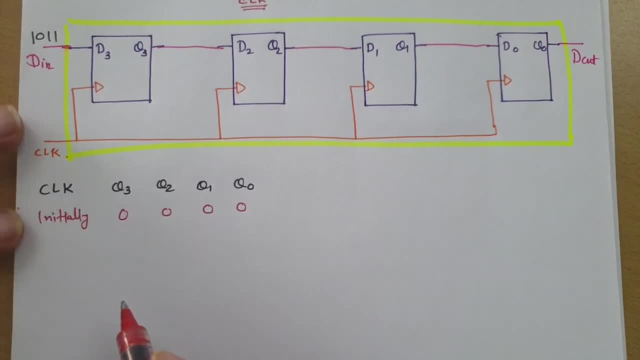 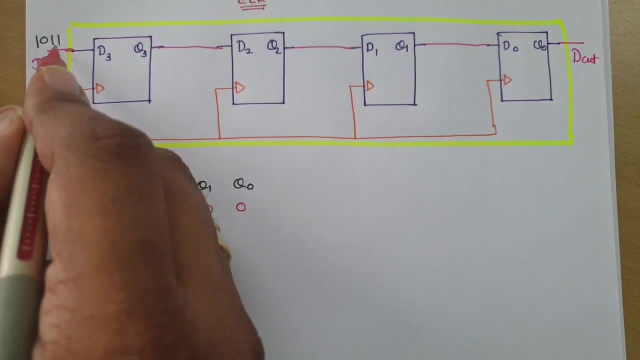 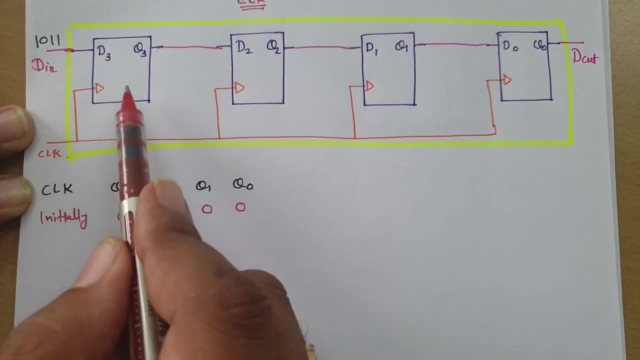 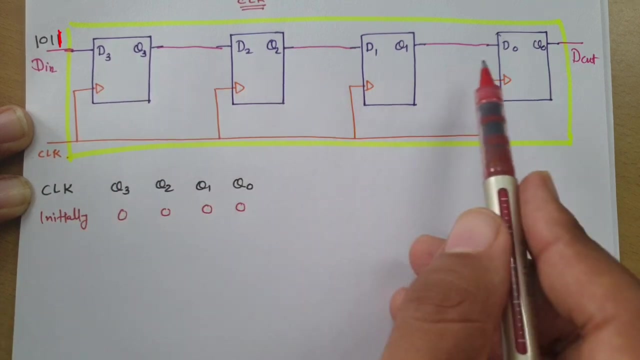 is zero. Now see 1011. that is what we are going to insert over here, So first we'll be inserting this one. Now, as for the basic working of D flip flop, as we give clock, what will happen? that input data that will go at output side right, so data that will shift in this. 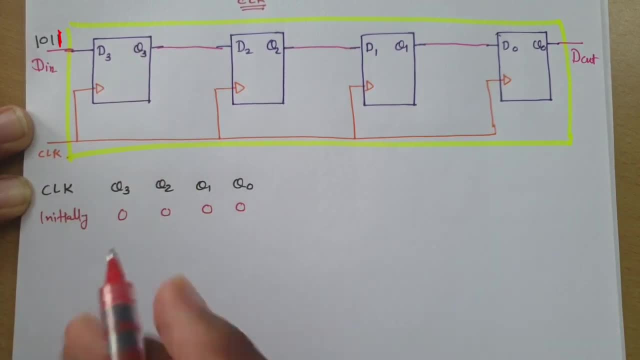 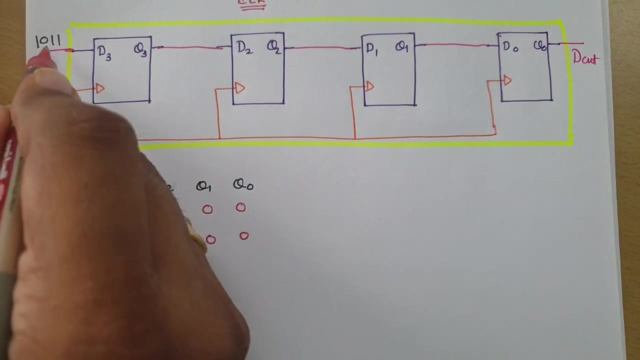 direction. so first one that will be appearing at Q3 after positive trigger clock and whatever data that was there previously, that will get shifted in this direction. so you see, this zero that will shift over here, this zero that will shift over here and this zero that will shift over here now when you give next clock. then this second one that will go at output. 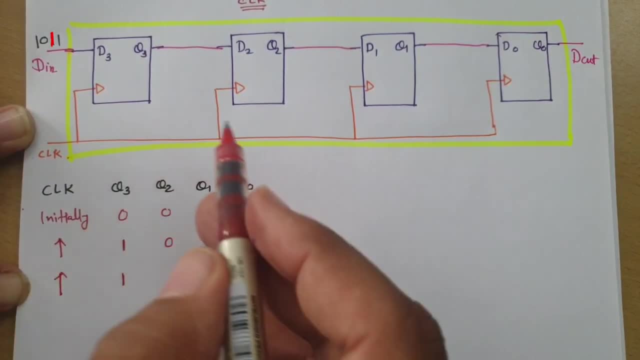 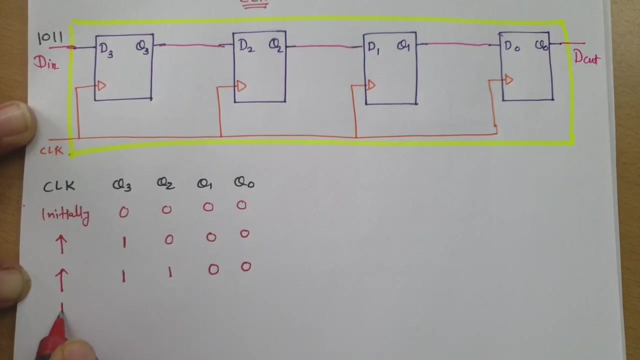 side, q3, and this previous data that will get shifted in this direction. so this one that will come here at q2, this zero that will come at q1 and this zero that will come at q0. now, in next clock, this third data, which is zero, that will appear at q3, and previous data, 1100, that will get shifted. 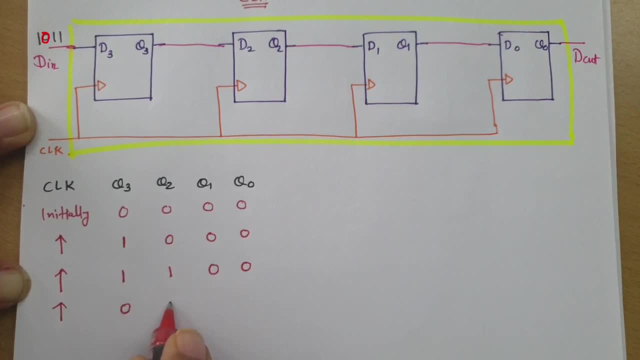 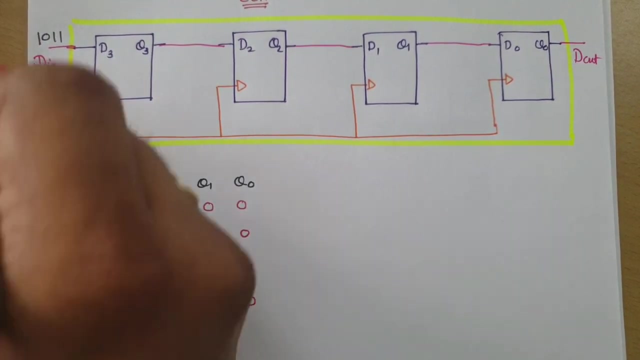 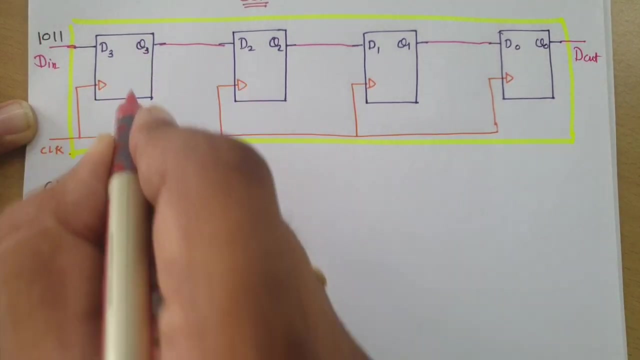 in this direction. so this one that will come at q2, this one that will come at q1 and this zero that will this, this, this, this, this zero that will shifted over here and as, if you give one more clock, then this fourth bit that will come at q3. so that is one and previous data that will get shifted. so this zero now. 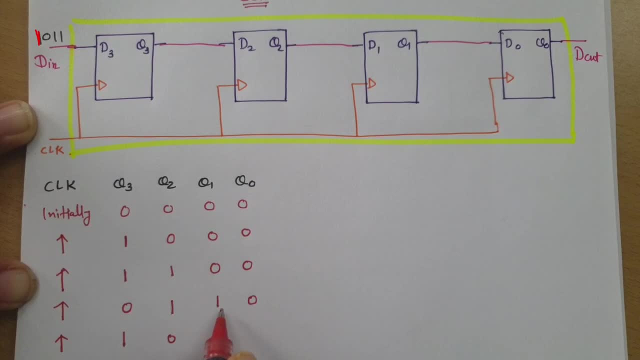 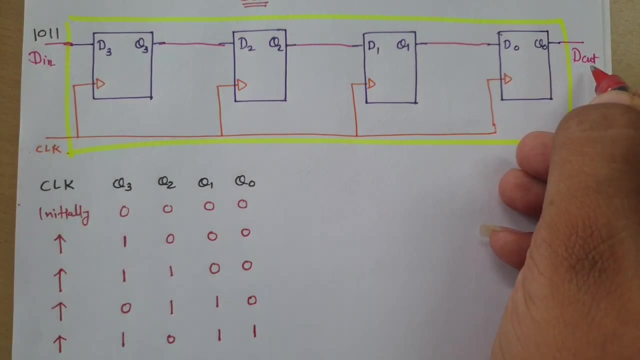 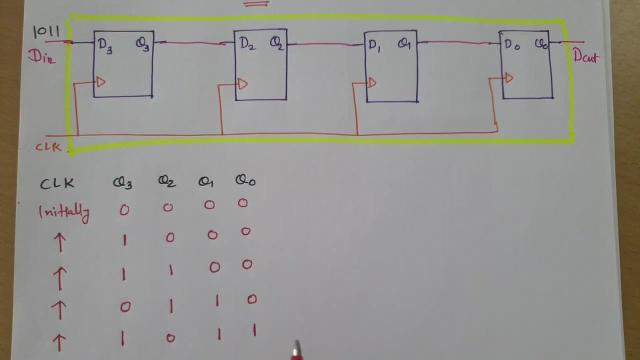 that will come over here at q2, this one that will come at q1 and this one that will come at q0. so this is what my first bit output, which is appearing at d out. but you observe, this is what 4 bit shift resistor right and after 4 clock, we are storing 4 bit data in. 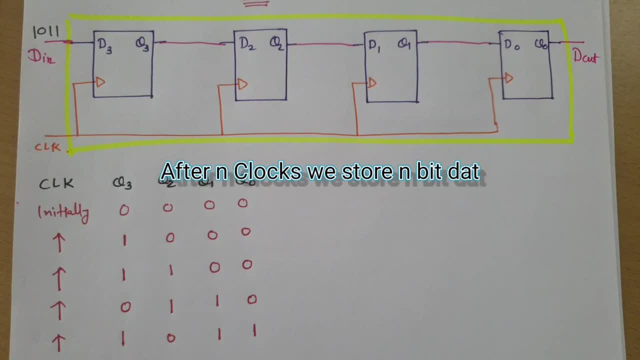 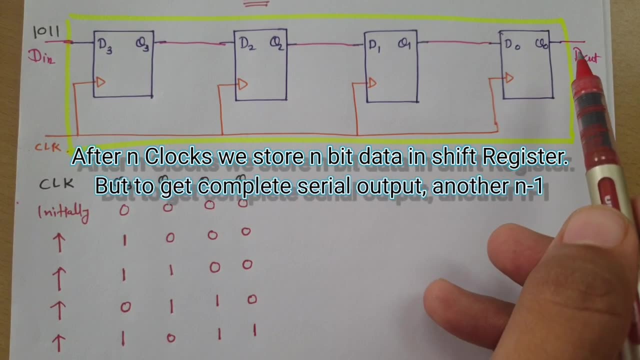 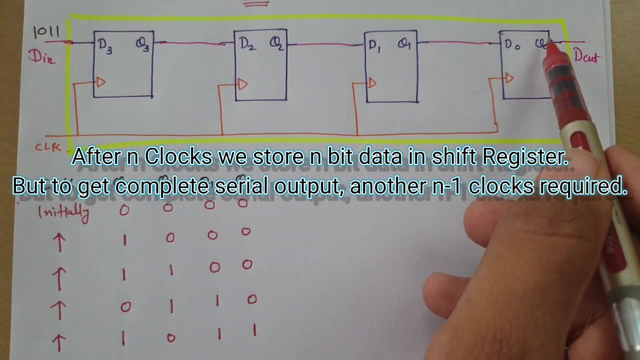 this shift resistor so we can say, to store data, n number of clocks are required. right, but here you don't have complete output. Our complete output, Our complete output, is 1011. so another 3 clock which is required so that at q0 you 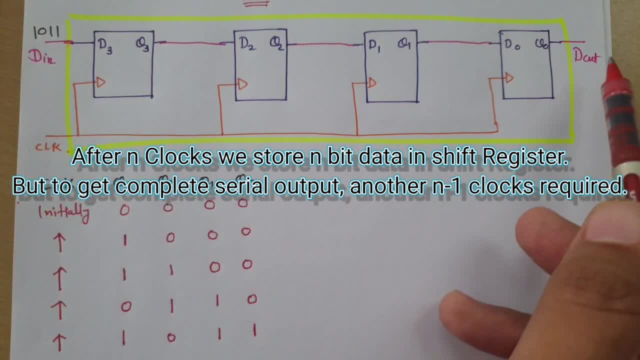 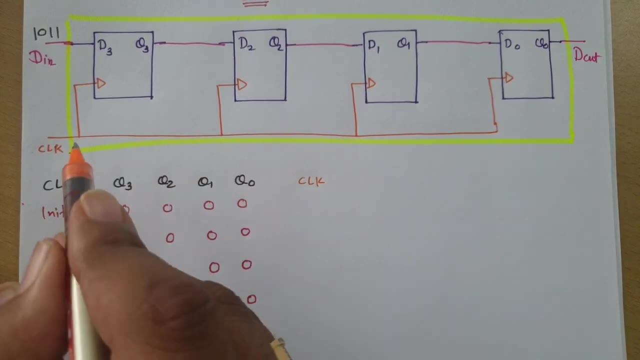 will be finding this 101 at d out serially right, So let us try to understand this by waveform so it will be more clear. So here I'm going to draw clock first, and here this is what positive edge trigger flip flop which we are using. 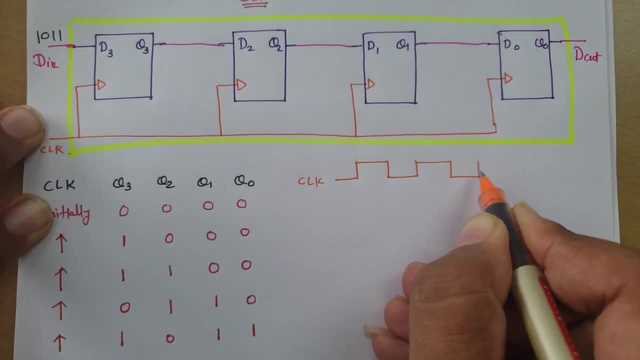 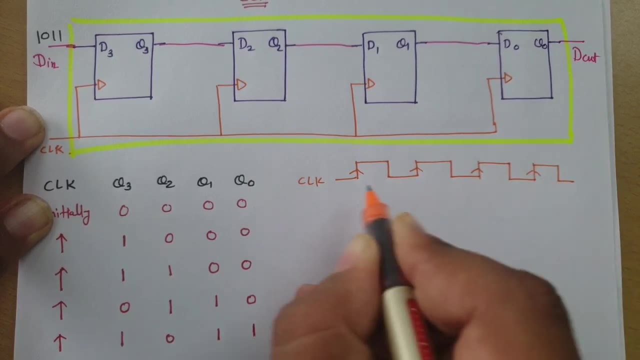 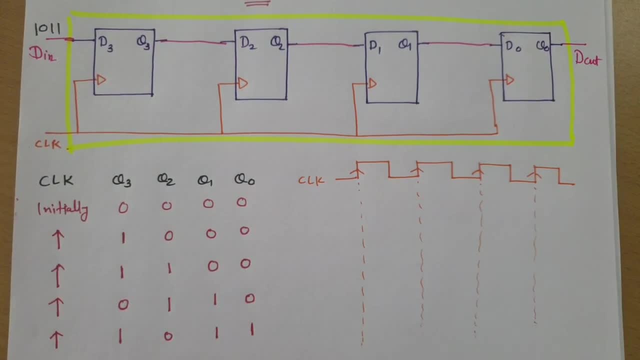 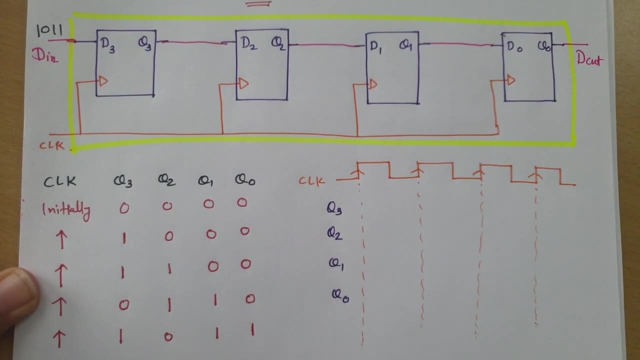 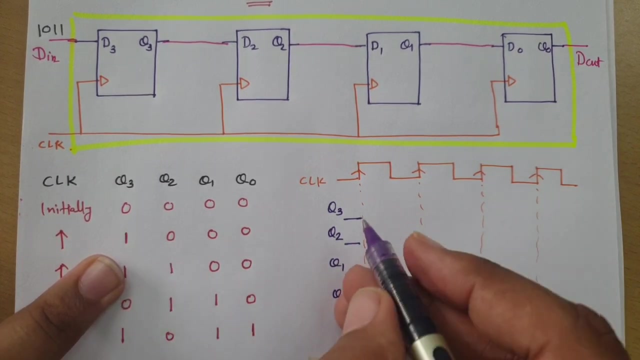 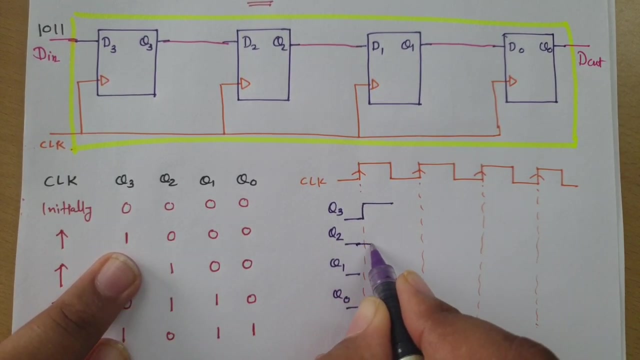 this line. Now, here we have q3, q2, q1 and q0 right, and initially that is zero, initially that is zero after first clock. After first clock, you see, data will be see. q3, that will become 1 right. q2, that is 0 only. 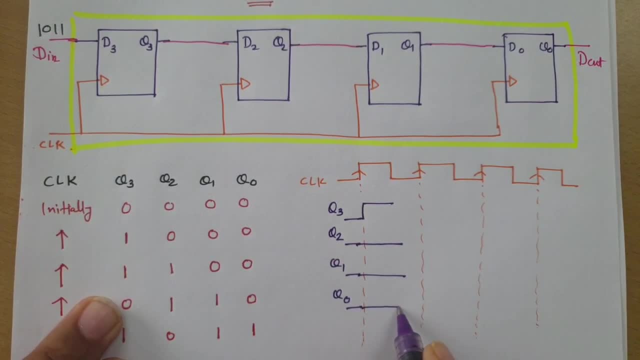 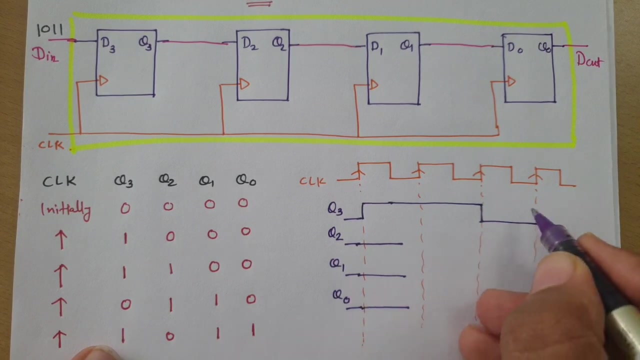 and q1 is even 0 and q0 is even 0. After second clock you see q3, that is 1 again. and then after third clock, q3, that is become 0. And after fourth clock, q3, that becomes 1.. 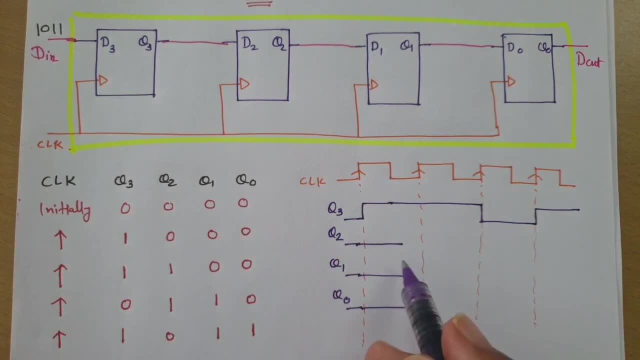 For q2. you see this waveform that will get shifted by 1 clock and we can plot it even see: after 0 there is 1, 1 and then there is 0. So this waveform, that is 1 clock shifted version in this direction. now you see q1, so that is. 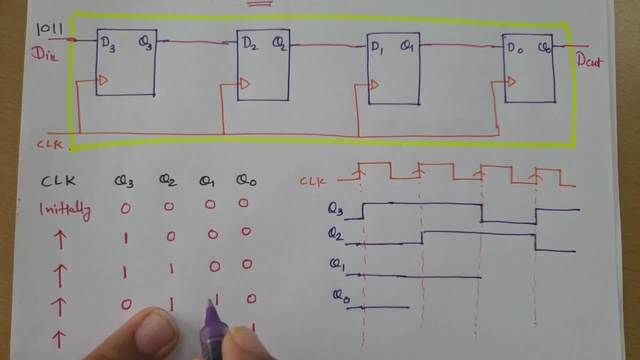 00.. And then 1: 1.. So that is again 1, clock shifted of q2 and if you see q0, so that is 000 and then 1.. And here we can clearly observe: initially this state is 0000 and with respect to clock, 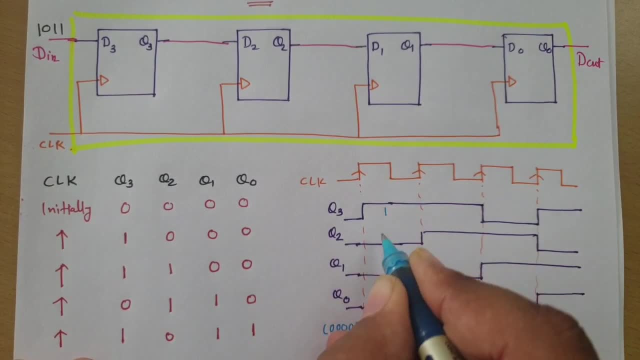 you see now q3.. That becomes 0. 0. 0, 1. 0. 0. 1, 0. 0. 0. 0. 1, 0.. 2, 0. 0 and after second beglock it is 1 1 0 0.. 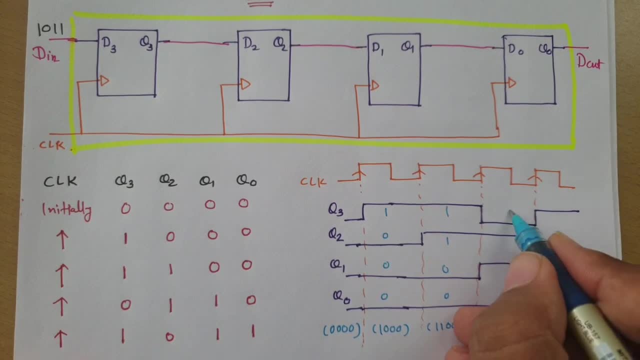 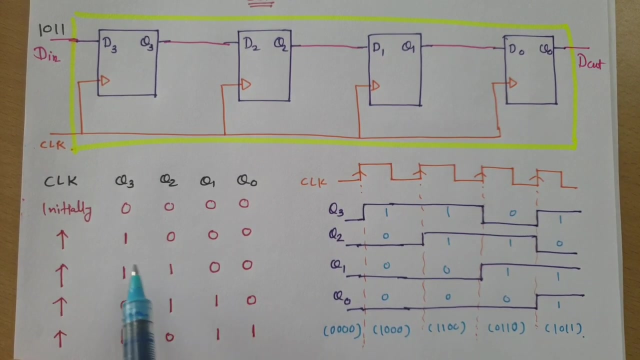 1, 1, 0.. 0.. After third clock it is 0 1 1, 0.. If after fourth clock it is 1011.. And you can verify it even. you see, After first clock it is 132.. 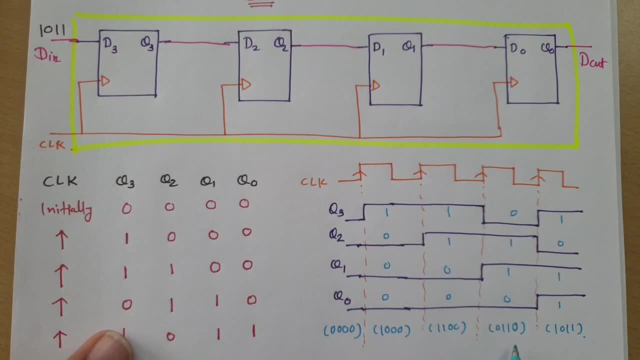 After 2nd clock it is 1100, after 3rd clock it is 0110 and after 4th clock it is 1011.. But this is not our complete output. Our output is Q0 only. So let me explain you generalize form. 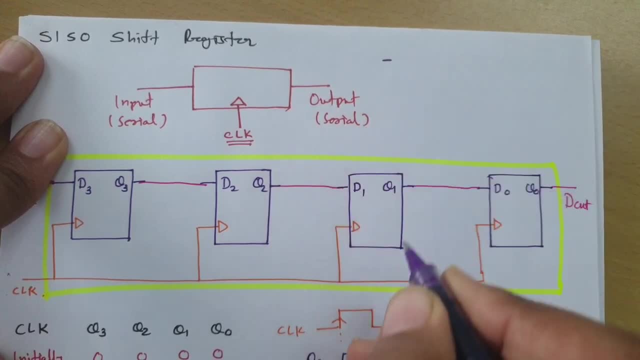 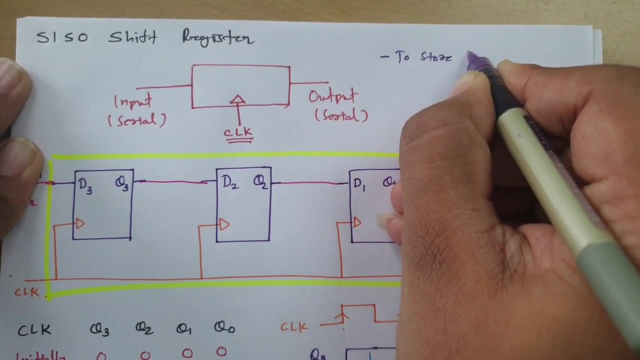 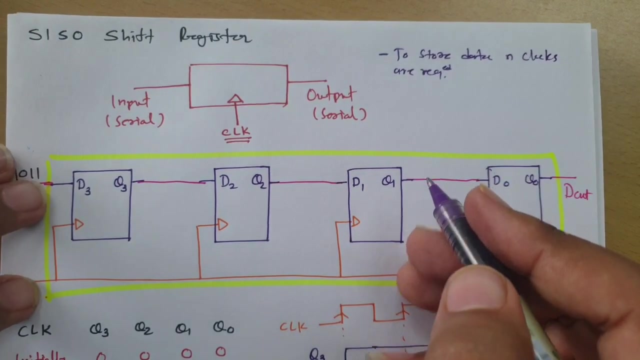 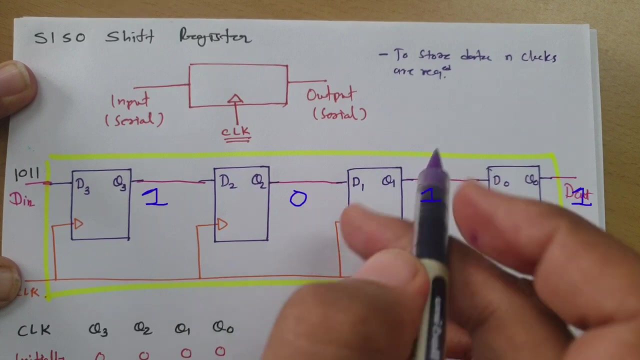 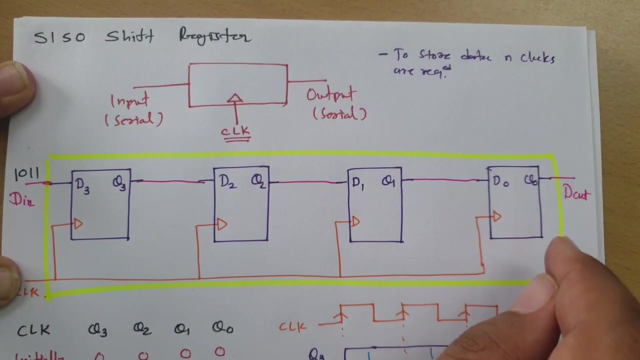 So see, to store we need n number of clocks. To store data, n clocks are required. Now you see, after 4 clock here we have stored complete data. So in general we can say n clocks are required to store data. But to get complete output additional n-1 clock is required. 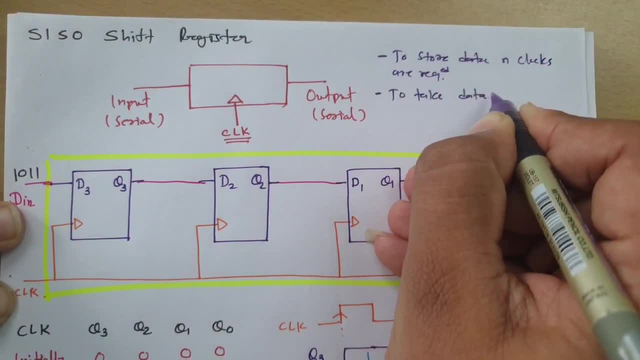 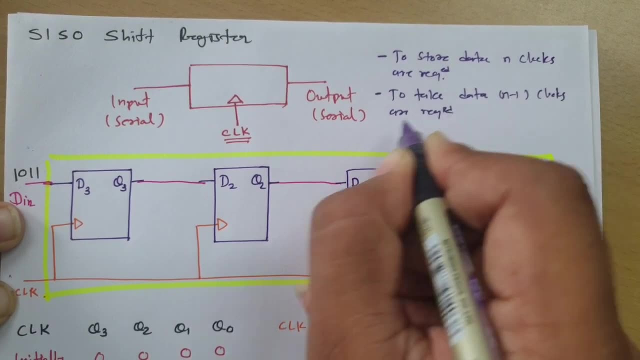 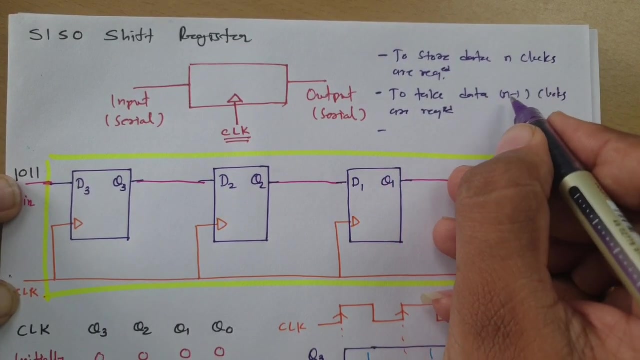 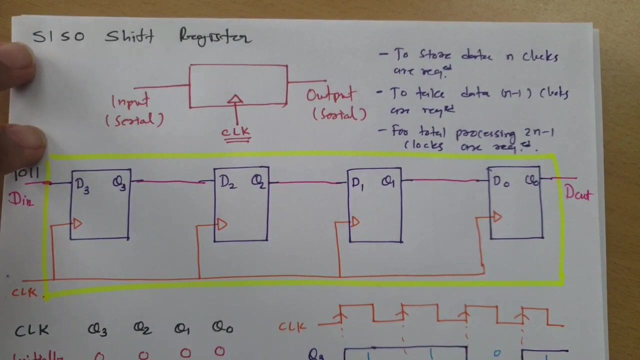 So we can say: to take data, n-1 clocks are required. So in general we can say: for total processing n plus n-1 means 2n-1 clocks are required. So in serial input, serial output, for total processing of data 2n-1 clocks are required. 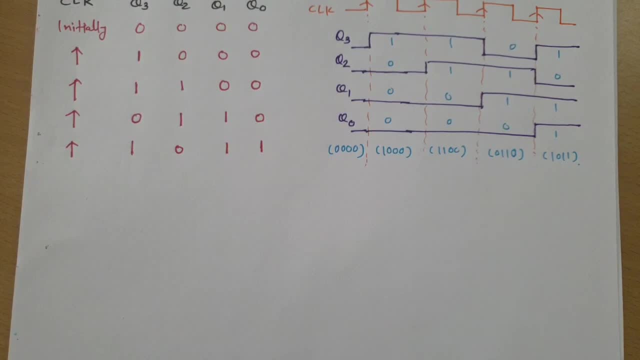 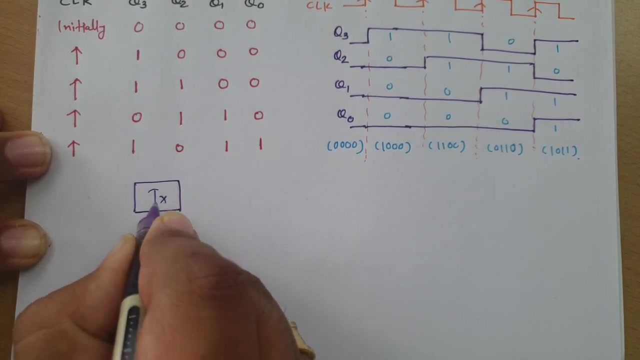 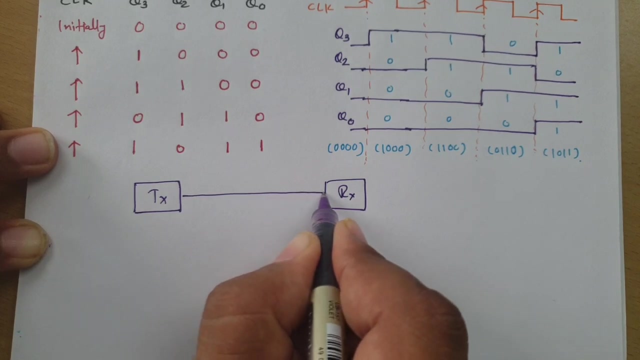 Now here, let me give you basic application which is there, with serial input, serial output. So we use this serial input, serial output with long distance communication. So in that you will be observing, here will be having transmitter, Here will be having receiver, And see if you have serial input, serial output, then you will be finding for long distance. 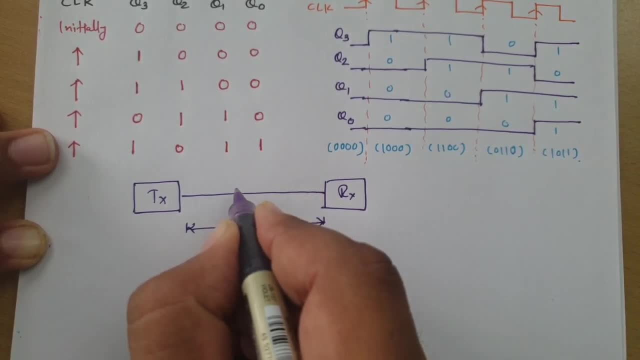 we can use this where, for example, if I say this is what we are using it for 1 kilometer, Then you see, in serial communication we just need one wire connection. But if you have parallel processing, Right So in that we need to have multiple wires connection. 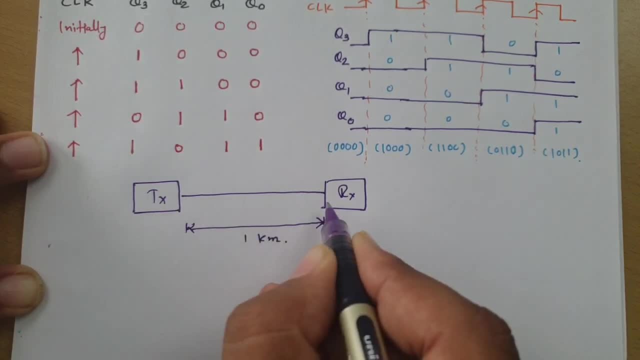 Like: see, for example, if you have four parallel wire, in that case cost of that metal will increase for long distance, Right? So here one can say: we use this for long distance communication. where wire cost, that we reduce, as single wire is required in between transmitter and receiver connection.